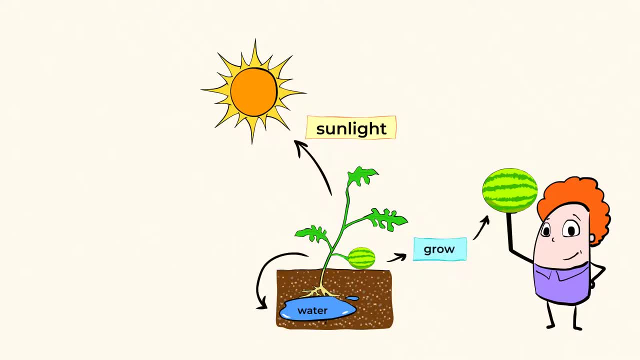 They're vital for plants to grow. Plants like watermelons essentially drink water and snack on the sun. Unfortunately, humans can't eat sunlight and we shouldn't even try to eat the sun. It's really, really hot, But plants can do it and that's what makes them so magical. 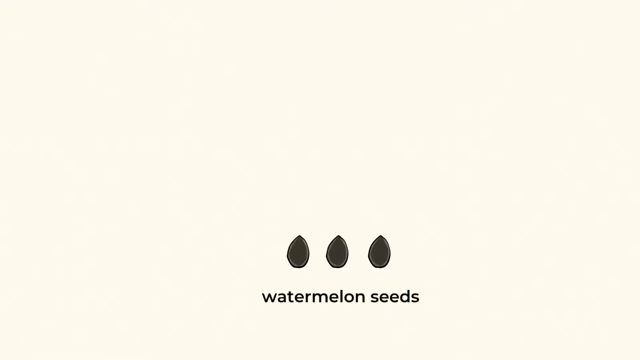 Now, if you get three watermelon seeds, you can use them for one delicious science investigation. So grab your magnifying glass and let's investigate the mystery of plants. We'll start with this question: Do plants need water and sunlight to grow? 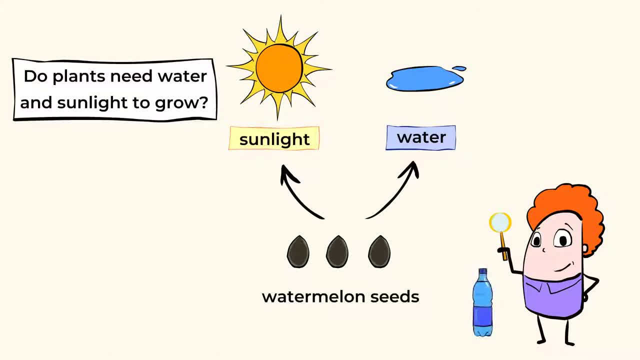 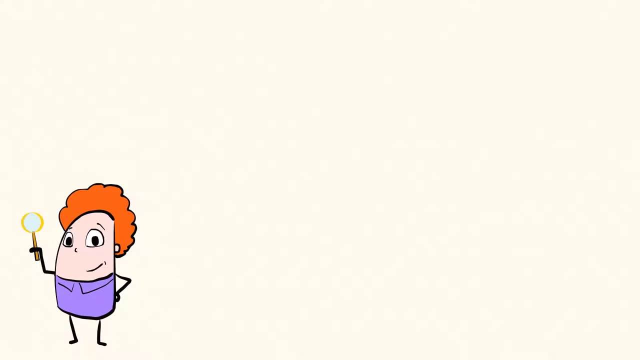 When you think about it even, you actually need water every day in order to stay healthy and grow, And you also need to go out and have fun in the sunlight. Do you think plants have those same needs? Let's find out. For this science investigation, we'll need three flower pots. 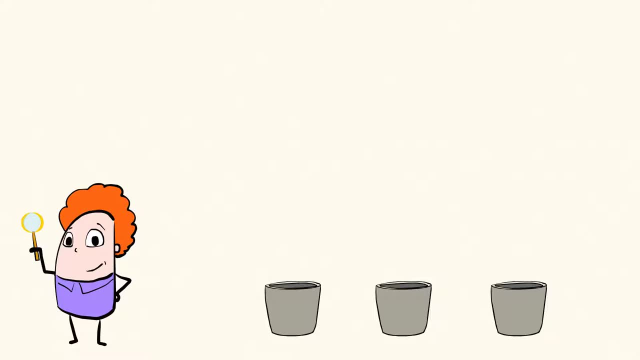 Do you have three empty pots at home? Don't worry if you don't. I've got a tree right here and I'm willing to share. But wait a minute, Is something missing? We can't just put the watermelon seeds inside the empty pots and expect them to grow right. 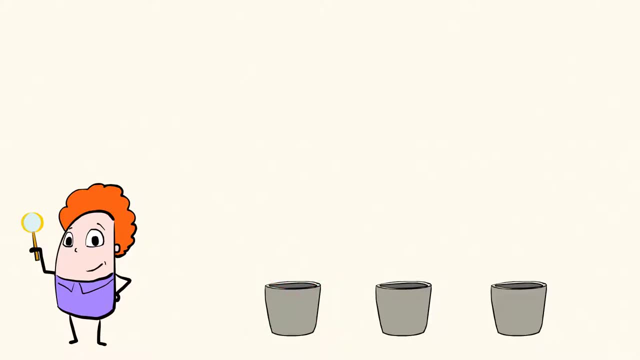 No, we can't. First, we need to fill the pots with some soil. Look at any tree, grass or flowers around you: They're all in the soil. And now that we've filled our pots with soil, we can plant the watermelon seeds. 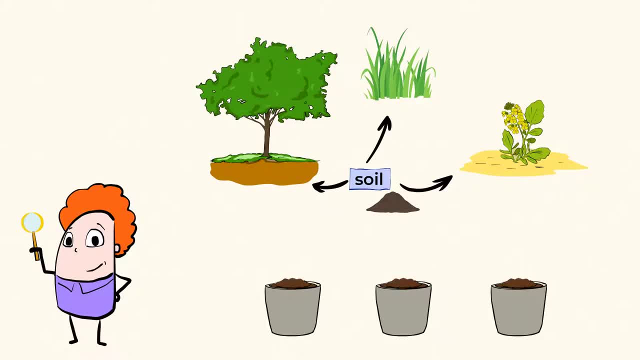 And then cover them with just a little bit more soil, Just like that. Add a bit of water for each pot And voila, We'll take one of the pots and place it outside in the sun, And we're going to water it every day. 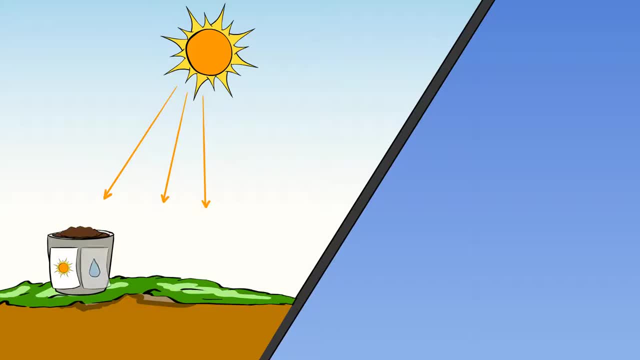 Now let's put two stickers on it, One with the sun and one with a drop of water, to indicate that we've watered this pot and left it in the sun. Then we'll leave another pot next to it in the sun, but we won't give it any water. 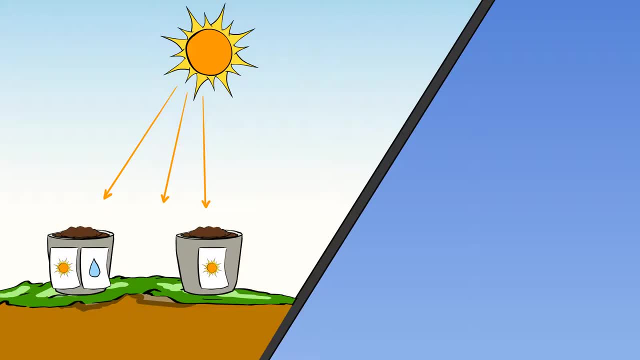 And so we're just going to put a sun sticker on this one, And the third pot will go inside the house, inside a dark kitchen cabinet with no sunlight, And we'll give it water but no sun And that means we're going to put just the water drop sticker on it. 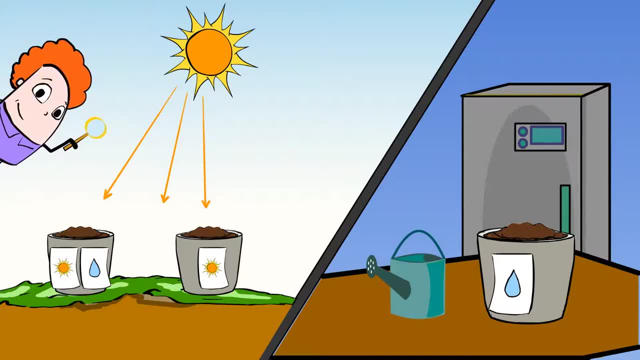 And now the investigation begins. What do you think will happen with the seeds in the different pots? Well, you'll have to wait for three weeks to find out, But luckily I have a time machine and we can jump into the future. So let's find out. 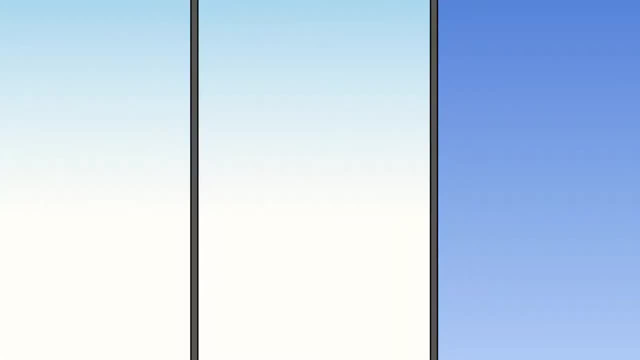 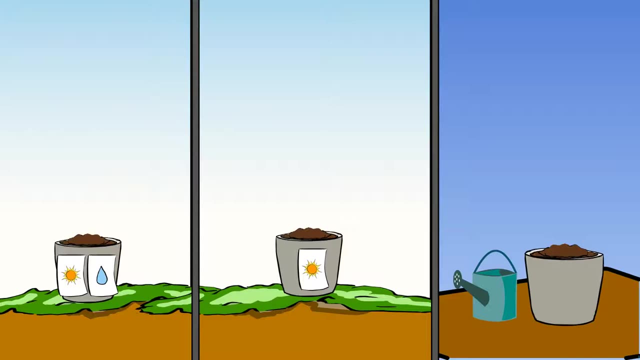 First let's examine the pots after one week. Now, have the different environments affected the seeds' growth? Well, the pot that gets both sun and water. it has a tiny root coming from the bottom of the seed. Now let's examine what's going on. 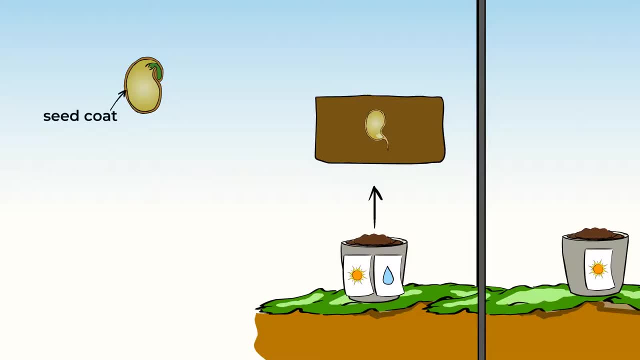 A seed has three, Three parts to it: An outer shell called a seed coat, An embryo, which is a baby plant, inside the seed, And endosperm- Endo-what. I know it sounds complicated, but it's actually just a fancy word. that means food for the baby plant. 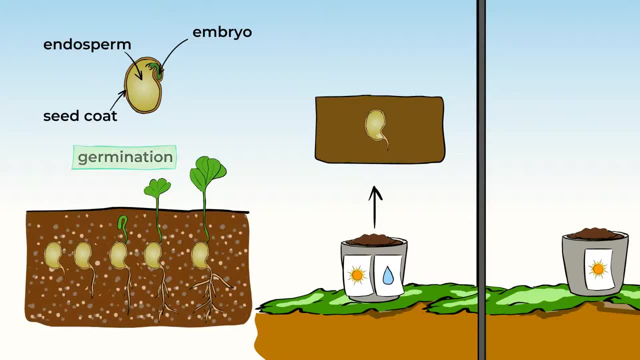 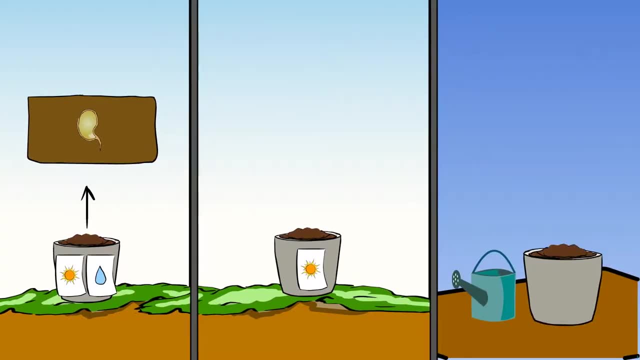 As the seed was planted in soil, it started its germination, Or in other words its growth and development, And the pot next to it. it didn't get water, since its initial soak also has a seed with a tiny root coming out. 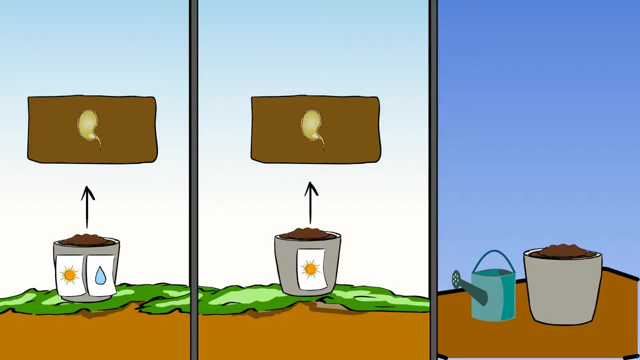 Oh, that's curious. Maybe water isn't that important after all, But this is only the first week. Let's not make any conclusions yet. Oh, and let's take a look at the pot in the dark cabinet as well. Whoa, look at that. 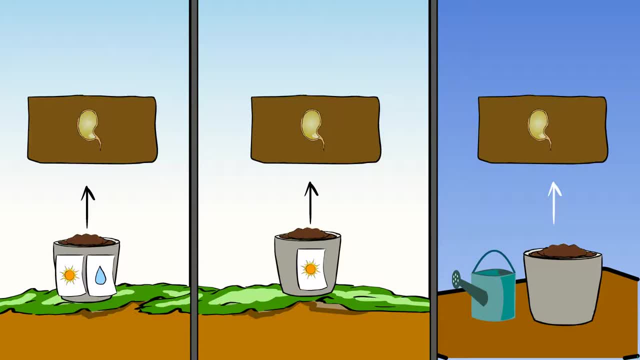 It has some tiny roots coming out too. What a surprise. Now all our seeds with their roots can take in water from the surrounding soil. Pretty cool, huh. Now let's check what happens after two weeks have passed. And here we are, two weeks later. 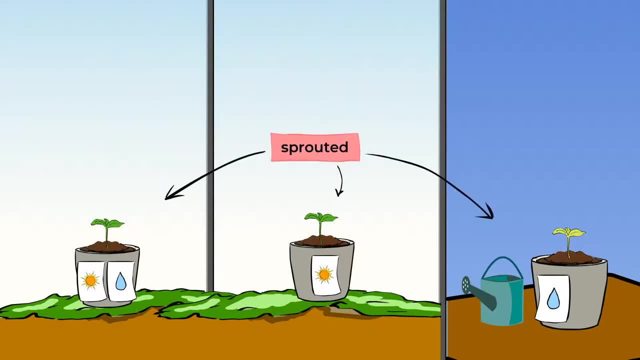 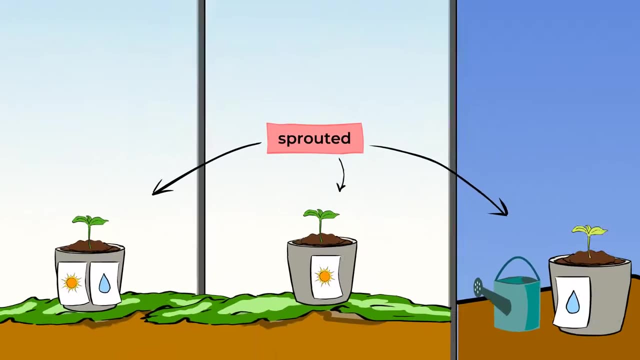 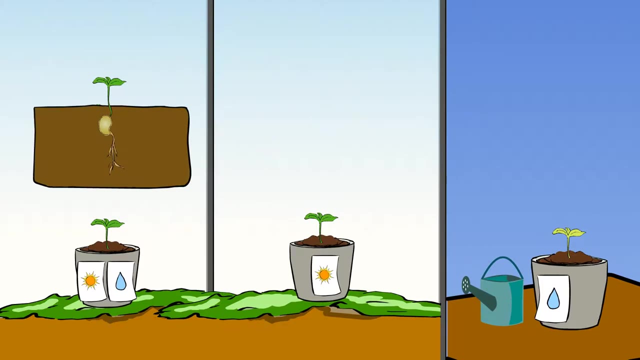 Wow, look at them, They've all sprouted. This means that a shoot with its stem and a few leaves has pushed the soil and come out. The plant that gets both water and sunlight is doing really well. It has more roots in the soil and a shoot with a little stem with some leaves above it. 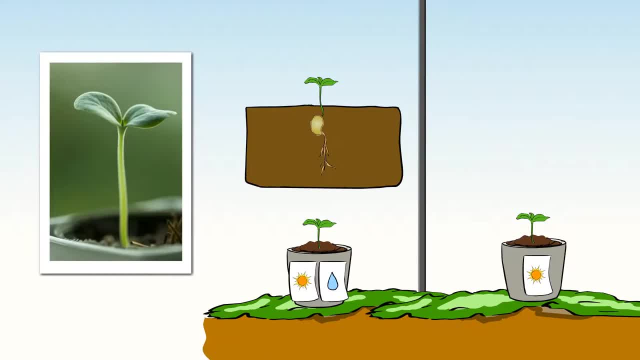 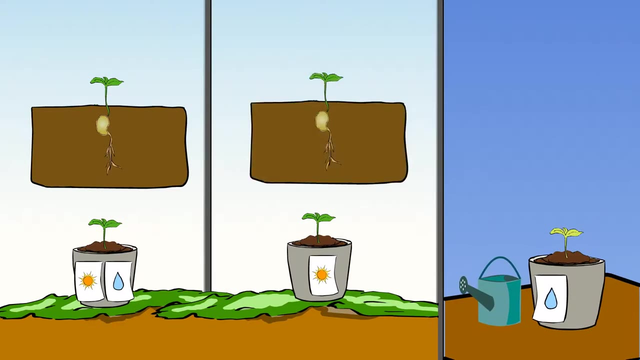 Can you see it? This part of the plant's growth is called the seedling stage, And this means that the watermelon is a small plant with some roots and a few leaves- And would you look at that? And the pot next to it, which doesn't get any water, also has a seedling. 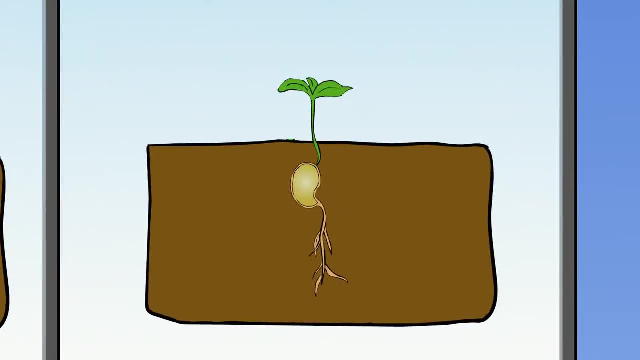 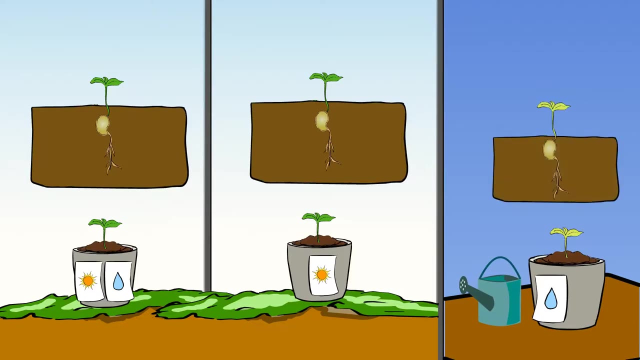 How interesting. The shoot tried to reach above the soil and get sunlight and to grow a small stem, And that must be because of its hidden food supply, The endosperm. And what do you think happened in the dark cabinet? Well, let's take a look. 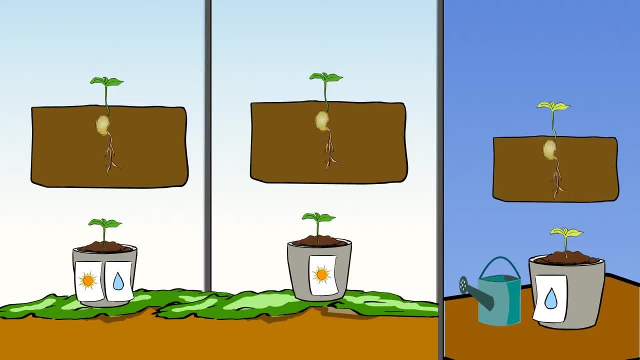 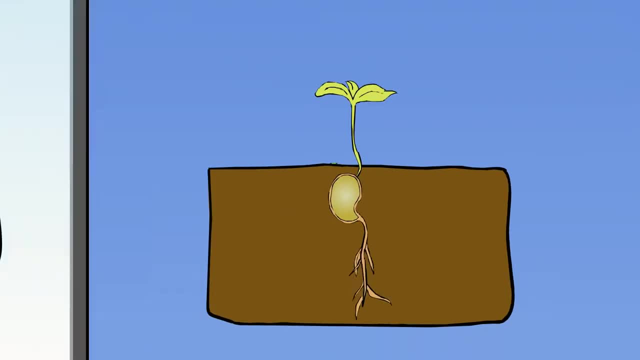 Oh, wow, The seed that didn't get any sunlight is growing faster than our other seeds, But the stem is a bit yellow. Oh, these results have befuddled our brains. You know what? I think we need to jump ahead to the third week. 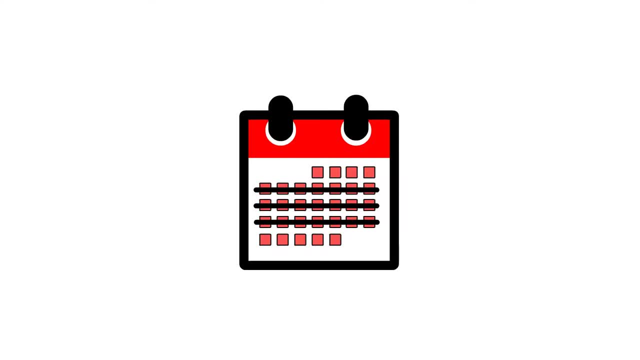 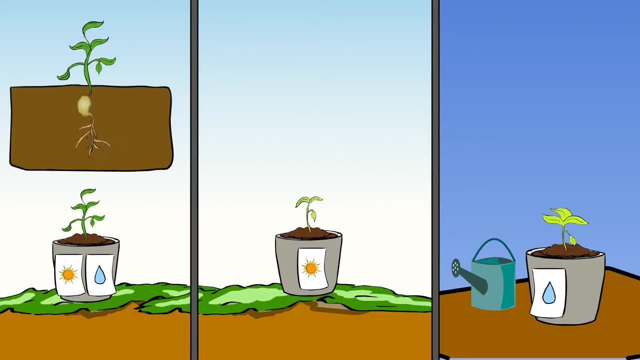 Now let's look ahead into the future and let another week pass. After three weeks of sun and water, the seedling in the pot that gets both sun and water is still thriving. It's developed more leaves and the stem has grown taller and thicker. 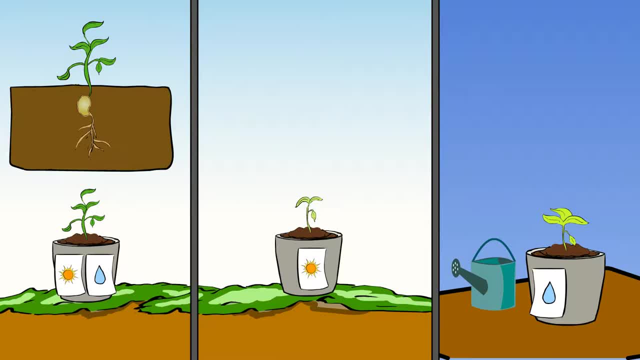 The roots are longer and stronger than the week before And our plants in the experimental conditions- no sun or no water- still continue to grow. But did you notice? These plants seem to have thinner stems, fewer leaves and lighter colors, And that's because just water or just sunlight doesn't give them enough energy to grow. 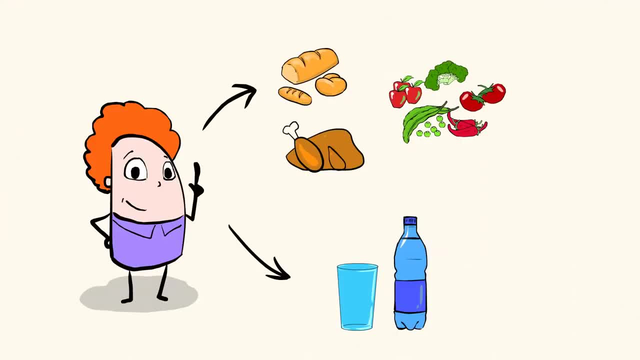 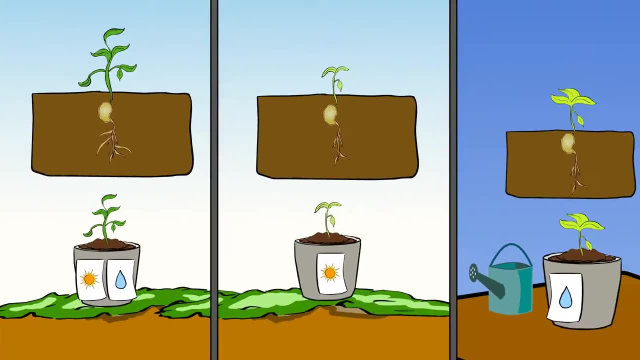 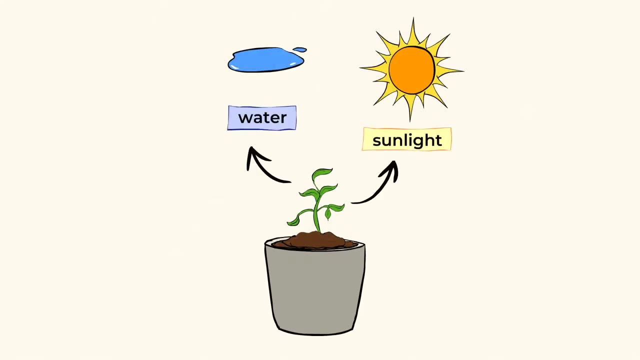 Imagine it like this: You need to eat and drink water, right, You can't just choose one, or you'll either be thirsty or hungry. Well, plants are like that too. Our investigation shows that plants need both sunlight and water in order to grow. 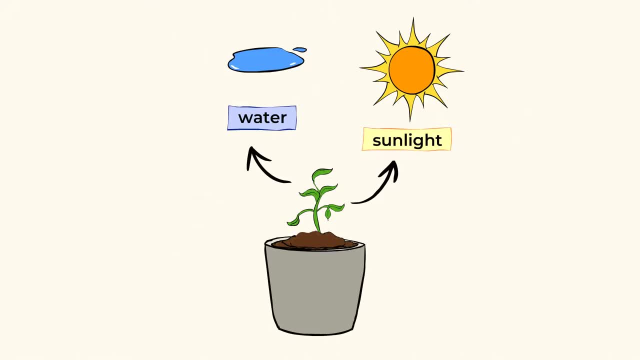 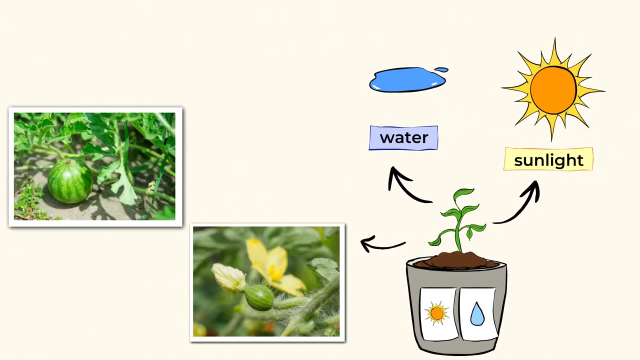 Plant seeds are smart and mighty. They know what to do when they receive water and sunshine. The seed that survived used water and sun as food, And it won't stop here. This little plant will keep growing into a bigger and bigger plant, And do you know what will happen next?